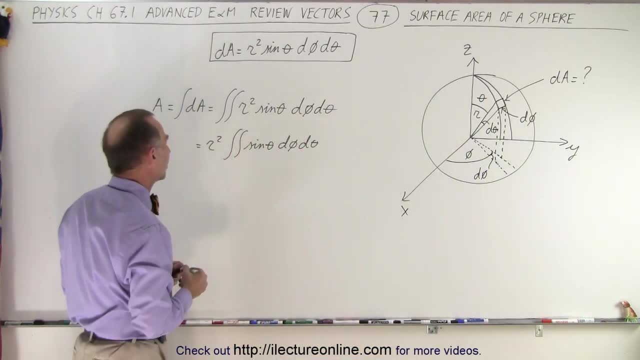 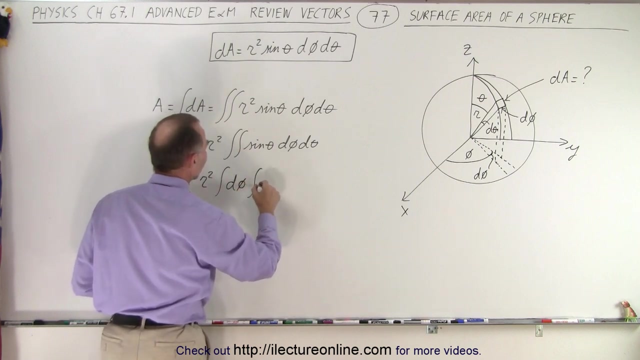 all the way around the circle to get the full surface of the sphere. So this looks as follows: This is equal to r squared times the integral of d theta. Oh no, no, Let's go. d phi, Let's make this. d phi times the integral of sine of theta. d theta, Let's just. 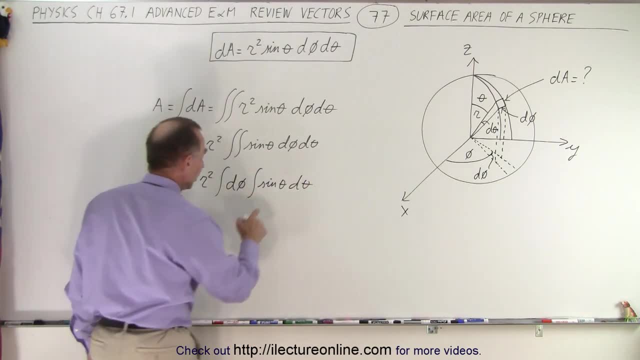 do that. It doesn't matter what the order is that we do it in. We could do it in either order. So theta will go from 0 to pi and phi will go from 0 to 2 pi. So let's do this one first. 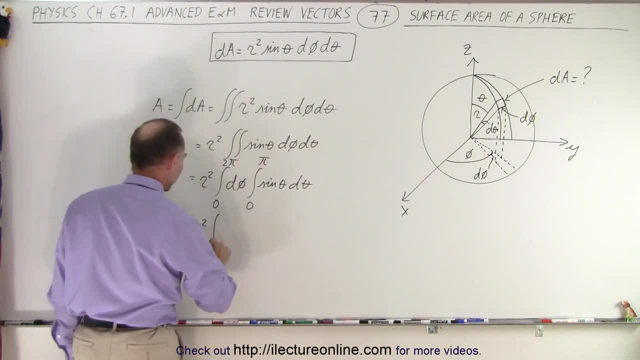 So this is equal to r squared times the integral from 0 to 2 pi of d phi times. Now, the integral of the sine of theta is the negative cosine of theta, Negative cosine of theta evaluated from 0 to pi, which is equal to r squared times the integral. 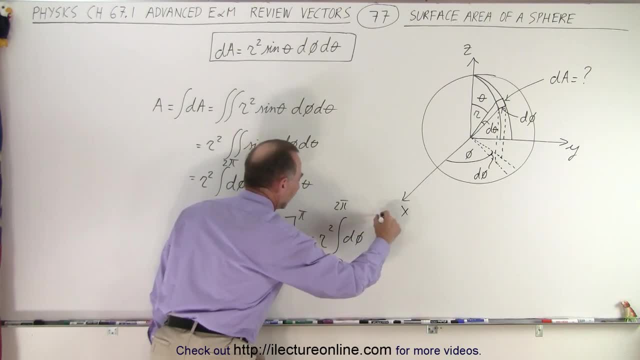 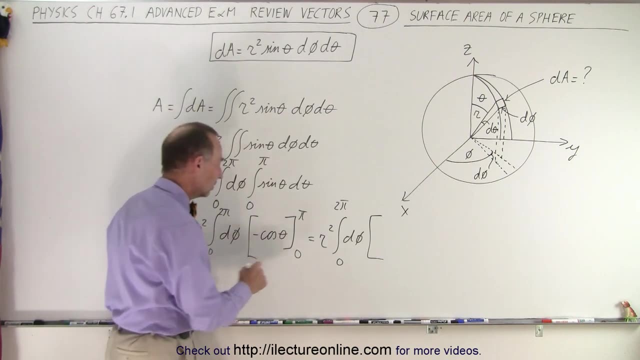 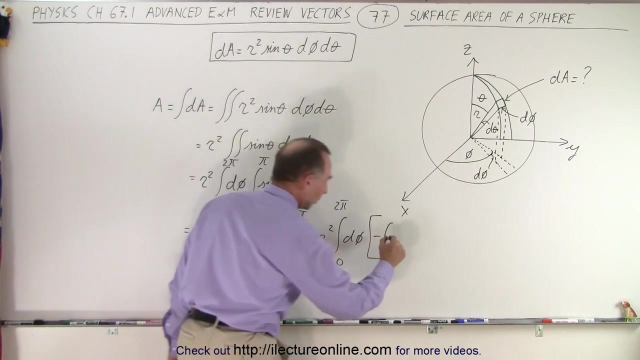 of d phi from 0 to 2 pi And then we multiply the times when we plug in the upper limit. Now the cosine of pi. well, let's see here, Let's put a negative like this So we don't get confused with the sine. So I pulled out the negative. The cosine of pi is a negative 1,. 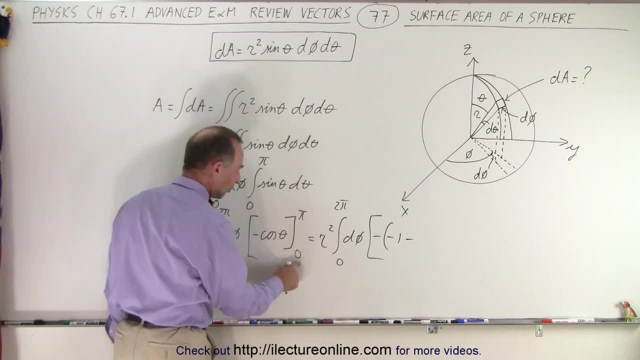 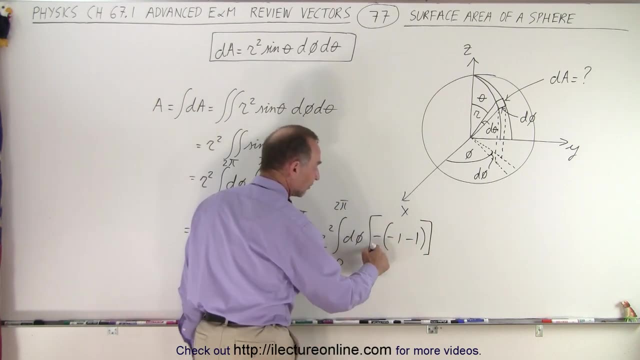 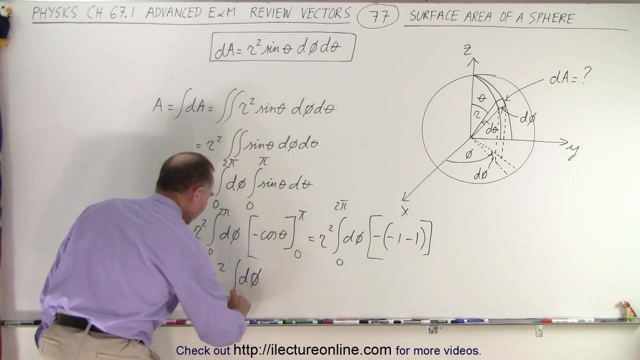 and we subtract from that the cosine of pi of zero. now the cosine of zero is one, but we're subtracting it so that negative one again. so we have a negative one, negative one that's negative two times, the negative is positive two. so this becomes equal to two r squared times the integral of d phi from zero to two pi, so that when we 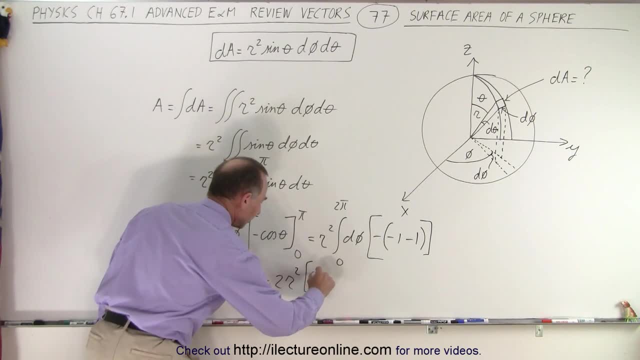 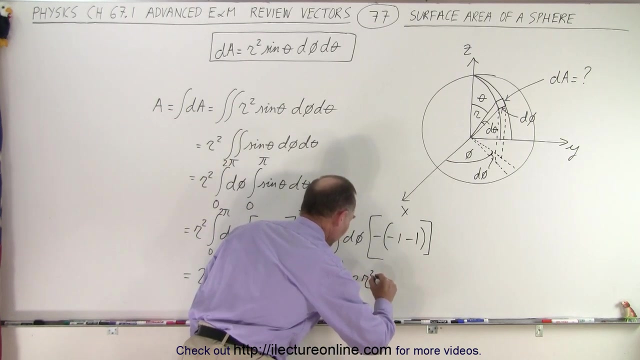 integrate that we get two r squared times the angle of phi from zero to two pi. so when we plug in the lower limit we get nothing. plug in the upper limit, we get two pi. so this is two r squared. that's a terrible looking r. let me try that again. r squared times two pi multiplied by times two. 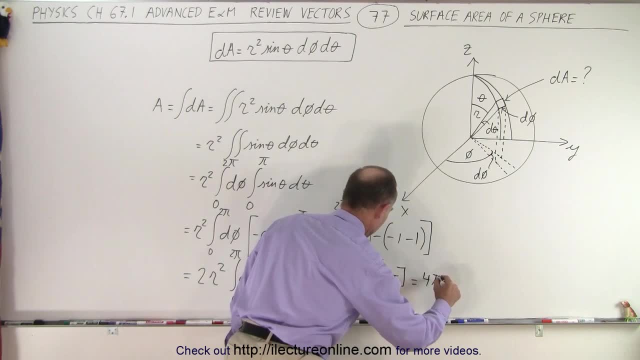 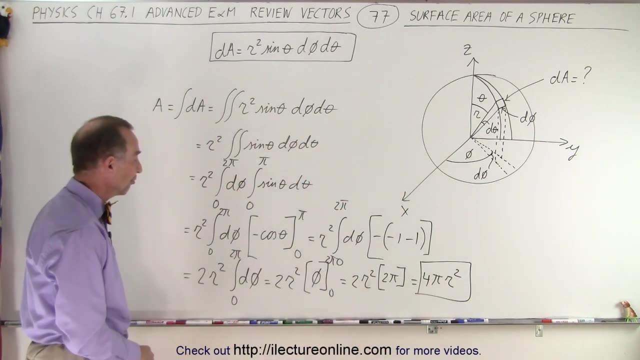 so we get four pi times r squared, and that is indeed the surface area of a sphere. so that's how we apply the definition of the d? a: a surface element on a on a sphere in spherical coordinates. then we realize that d? a is simply a double integral. 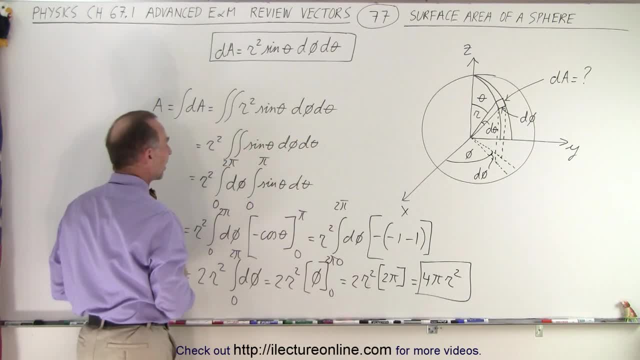 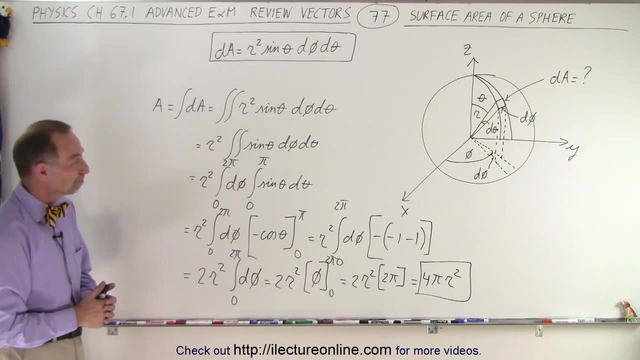 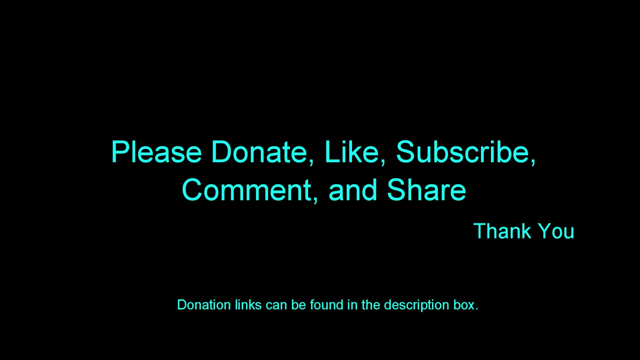 over theta and phi r becomes constant, so it goes outside and then the rest. you just follow the methodology and that is how it's done you.